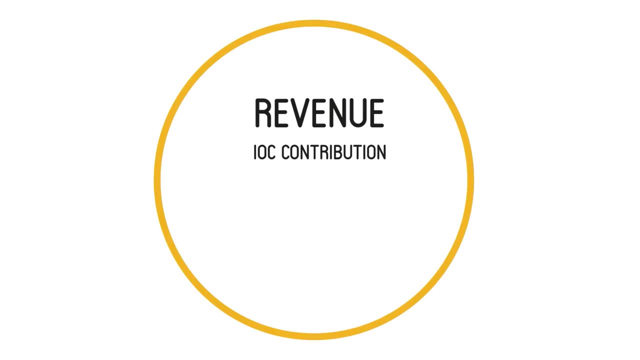 But by the revenue coming into the Games, the contribution of the IOC and income from sponsors, ticket sales, Games merchandise and hospitality. Games organizers assume that the Games organization is the only organization that can support the Games organization. The benefits so far have broken even. 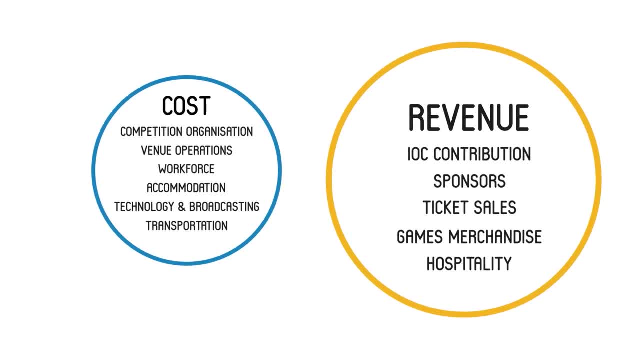 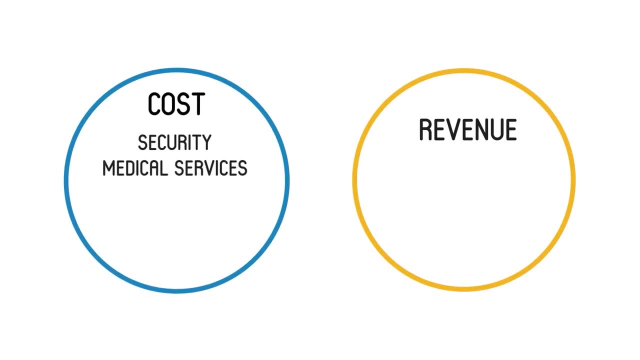 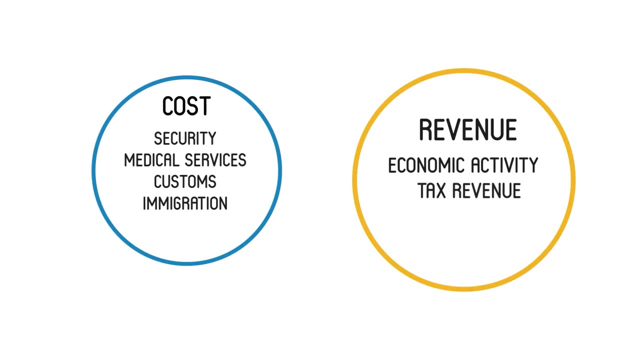 Some have made a profit, profit that is reinvested locally for the benefit of the city and its people, especially the youth. Public money is used for things like security and medical services, customs and immigration, But these costs are covered by the increased economic activity and tax revenue that's generated before, during and after the Games. 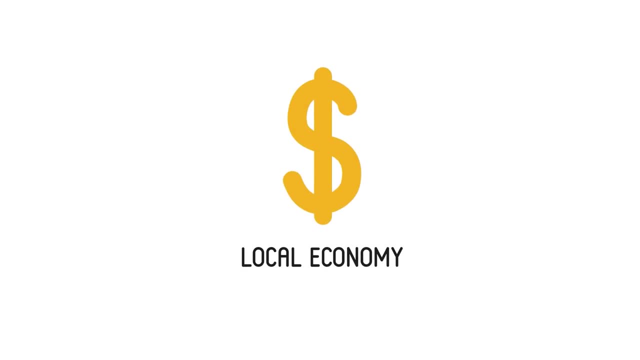 How does that work? Well, for example, Games organizers and and visitors spend money in the local economy. They employ local people and use local suppliers. Those people then also have more money to spend in local shops and restaurants, Local businesses, which in turn have more money. 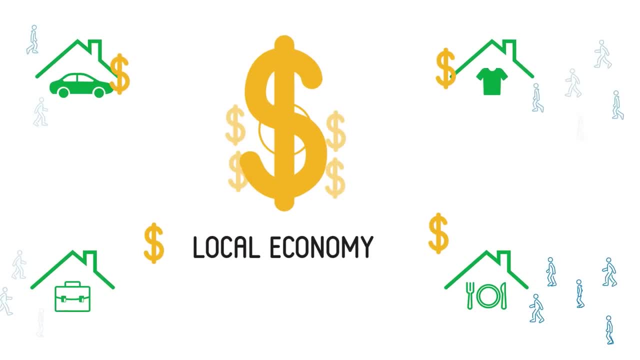 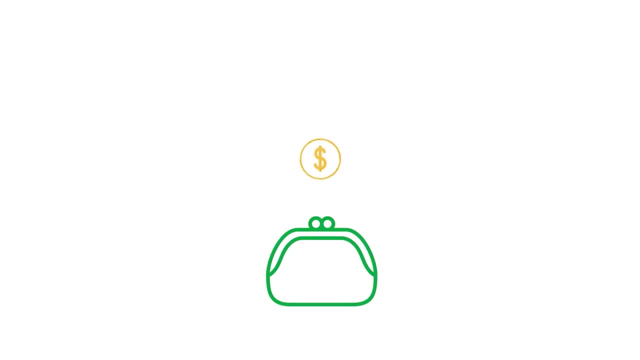 to go out and employ more local people. The ripple effect of the games goes on and on, And all that increased business activity ultimately creates more revenue from taxation, Lots more, several hundreds of millions of dollars that find their way back to the public purse. 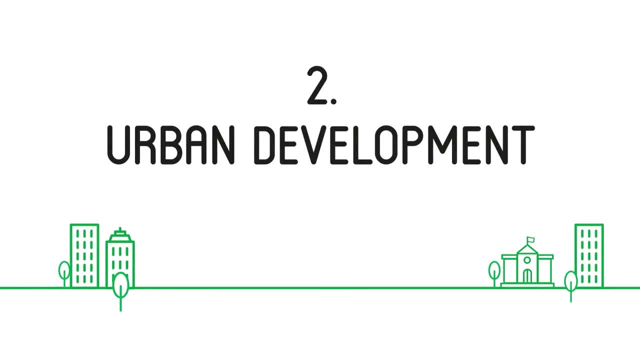 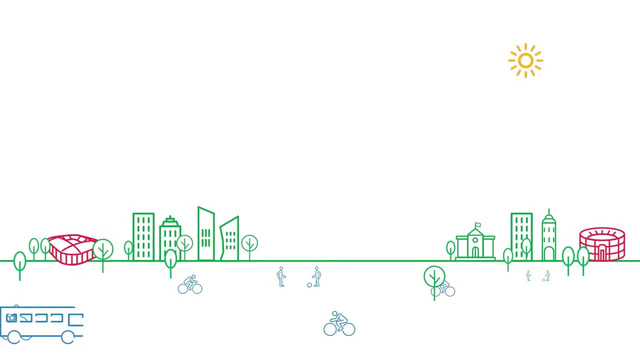 The second area relates to urban development. That's where things are now very different. The IOC has turned the page With the Olympic Agenda 2020, the new norm cities have full flexibility to find solutions without building venues and infrastructure they don't need. 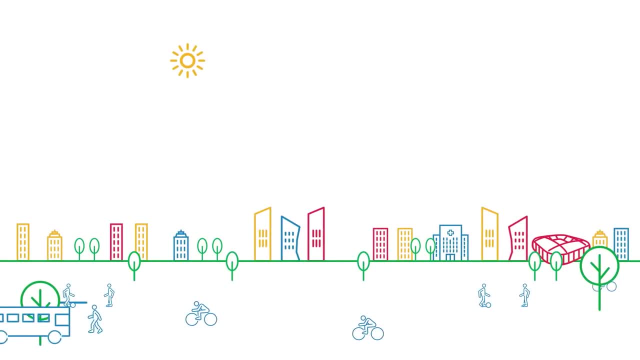 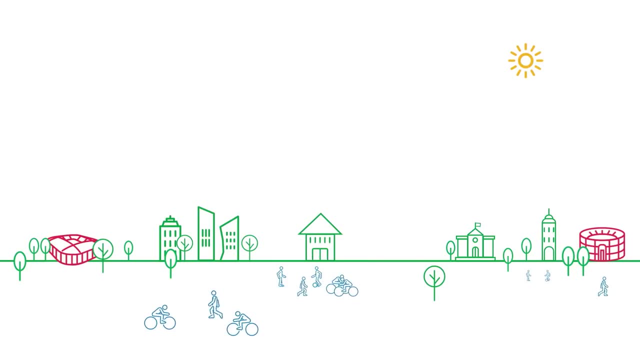 For example, they can use a venue in another city or city center to build a city, region or country. If anything is built for the games, it has to be part of an existing development plan, so it is useful to the city and its people in the long term. 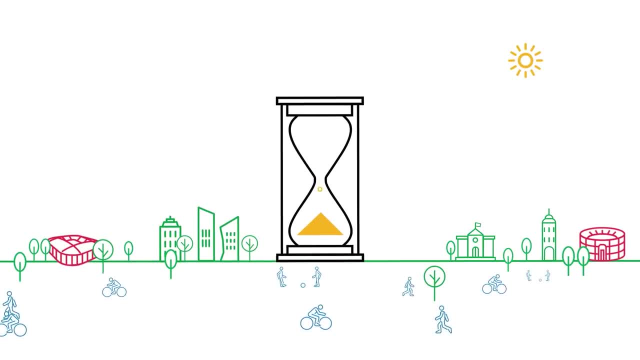 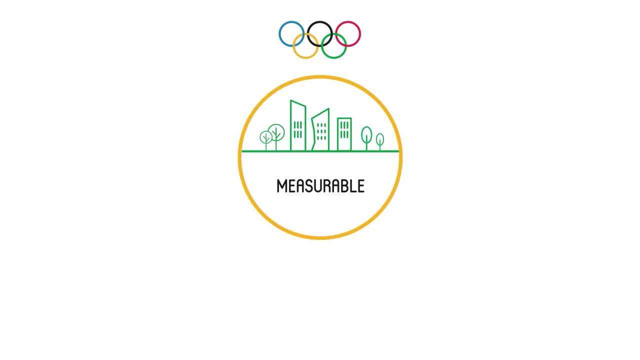 And, as we've just seen, that long-term legacy doesn't just come in bricks and mortar. It takes many different forms. The measurable: a huge injection of fresh revenue into the city through the workforce, employment, GDP and trade, and investment and tourism. 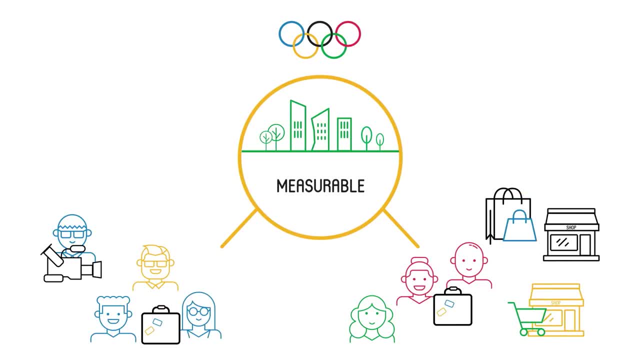 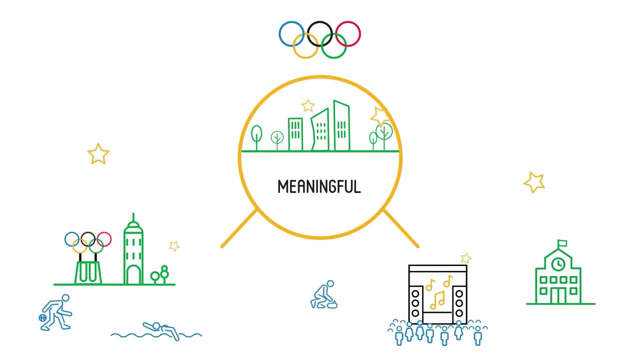 with more than $1 billion of revenue, Most of the money being spent in the local economy, The meaningful sport development, community cohesion, culture and education. venues being given a new lease on life, A workforce with new levels of experience and a city forever elevated.